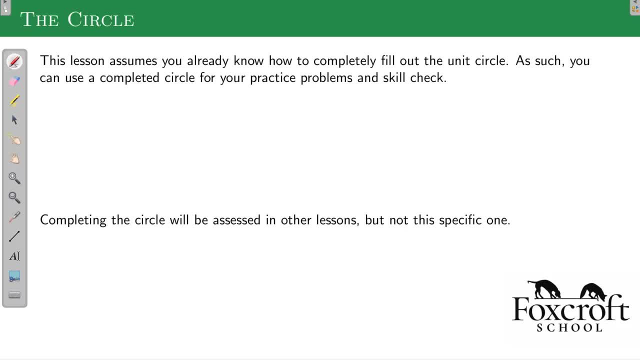 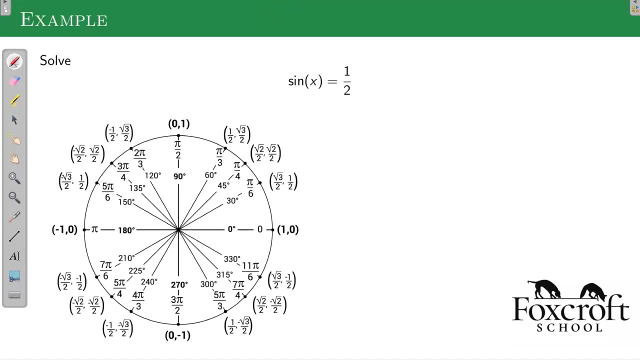 All right, so this lesson comes after you having to fill out the unit circle. So it assumes you already know how to fill out the unit circle, so you can use your unit circle for your practice problems in your skill check. For the test, you would have to recreate the unit circle anyways, and then you would use that unit circle for this. So for your practice, just pretend like you just fill out the unit circle, use the unit circle you've already done, and use that. All right, so the main thing we're focused on in this is not completing the unit circle, we already have it here, but we're focused on solving this equation. So this equation is sine of x equals one half. When is the sine of my angle one half? If I look at my unit circle, sine is y values, I see the y value is one half here, and the y value is one half here. 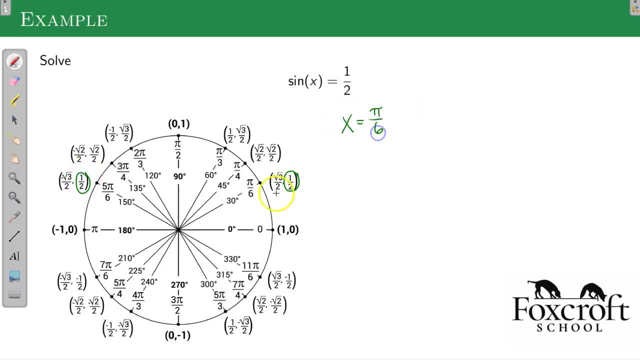 So x could be pi over six, that's that angle, or x could be the angle five pi over six. 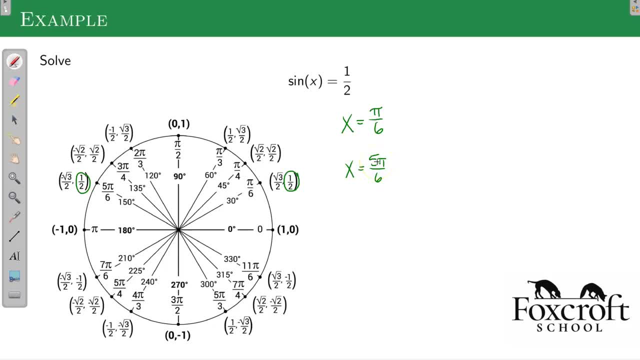 Okay, but unfortunately that's not the whole problem. That's actually really good, if you write that down you'd get a lot of credit. But there's a little bit more that's going on, because we know there's these coterm languages. I don't just have to rotate here and stop, I can rotate all the way around my circle and get that. So I'd also get x equals 13 pi over six, if I did an extra two pi. I can also do an extra rotation and come back around. I can also get, let's say I'm adding another 12 pi over six, 25 pi over six. Let's just do it one more time, for demonstration purposes. I could do an extra revolution and I could get 30, 37 pi over six. Yep, that's right, 37 pi over six. So all of these would all look like this pi over six angle, except for this one, this was on the left. And I could keep doing this. I could also go the opposite direction. I could do this, let's just erase some of this. I could do this, I could go around to here, that'd be negative five, negative 11 pi over six. 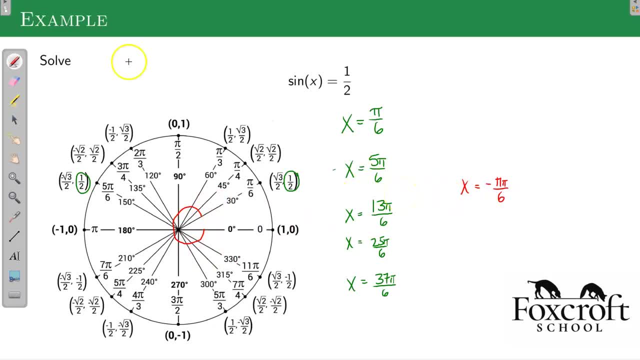 I could do it twice and get negative 23 pi over six and so on. So there's actually an infinite number of answers to these problems. And I don't want to write down an infinite number of things, it's not even possible. So what am I supposed to do? Well, there's a little shortcut for how I can write down my answers. I know pi over six and five pi over six are the kind of main angles I care about. But then I could also add or subtract two pi at any time. So if I add to this two pi times, just some random... Number. This will give me another answer. I can do the same thing here. K is just representing how many revolutions I do around the circle. But this is the notation we're going to use for these solutions. Our kind of starting angles are pi over six and five pi over six. And this plus two pi k thing, this is representing all the coterminal angles. 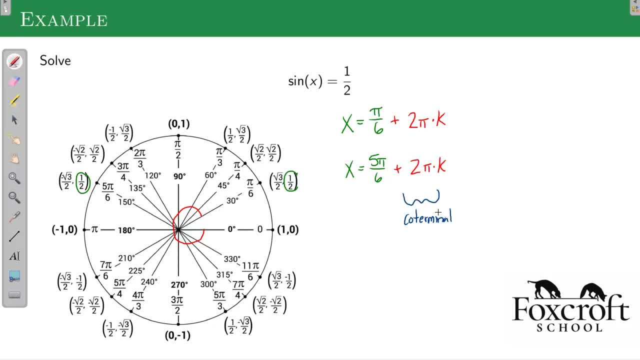 So really it's just this one extra thing. The unit circle will quickly give you the two answers. And you just have to remember there's one extra thing that you can actually get from the infinite number of answers. 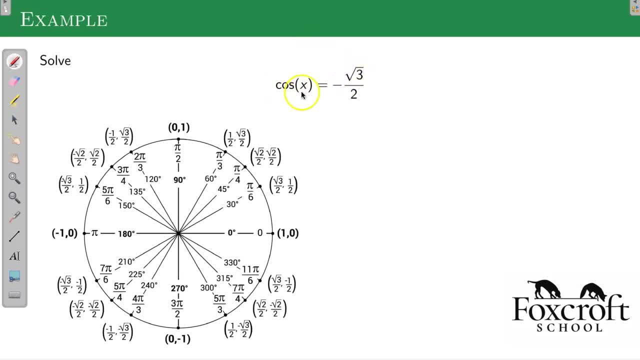 So what about cosine of x equals negative square root three over two? Cosine is the x values in the unit circle. So I'm trying to find when the x value is negative square root three over two. 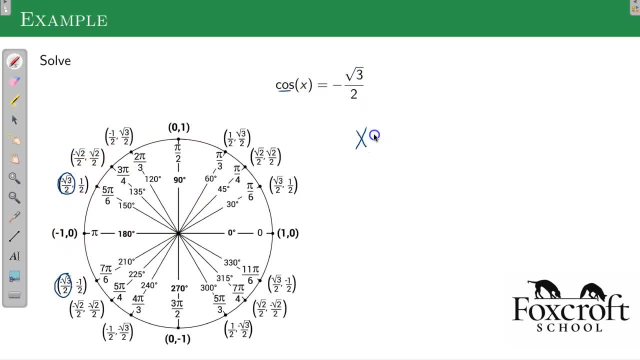 That happens here and here. So my answers are my angle could be five pi over six. Or my angle could be seven pi over six. 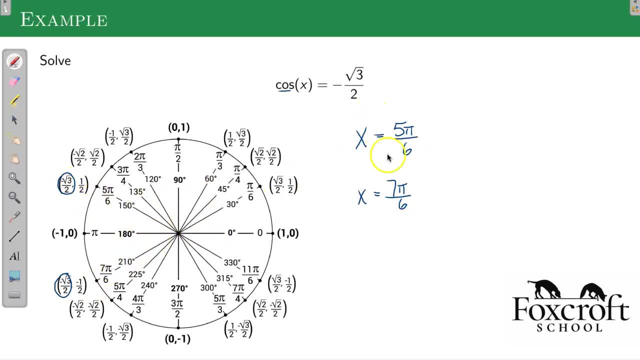 Those aren't the only ones. Any angle that looks like those could work. So I could also all these coterminal angles on as well. So there's an infinite number of angles, but I'm just kind of writing it in the shortest way it's possible to write those infinite angles. 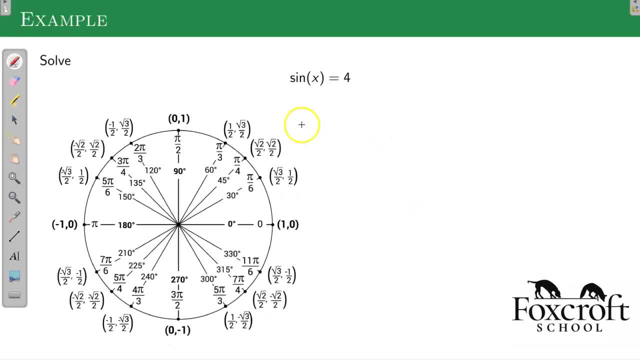 All right, what about sine of x equals 4? I can go around my unit circle and try to find the value 4 in the y position. You notice that won't happen. So what am I supposed to do? Well, if I think about my unit circle, if I go up to the top of my unit circle, that y value is 1. So 4 would be all the way up here. And 4 is never going to be on the unit circle because it's a number bigger than 1. So this problem just has no solution. The biggest that sine can ever be is at the top of the unit circle there is 1. 4 is bigger than 1. So this is always smaller than 1. This is 4. I get no solution.